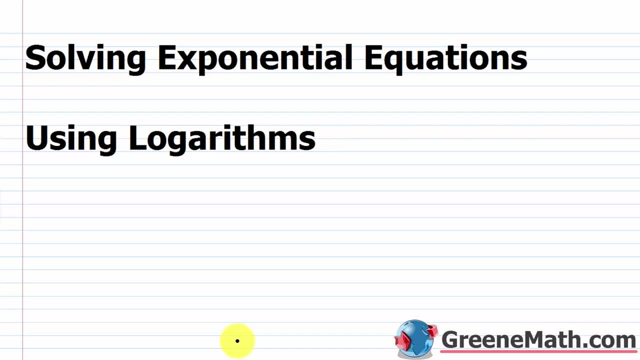 In this lesson we want to talk about solving exponential equations using logarithms. So at this point we already have all the tools that we need to solve any exponential equation that we come across. So I'm just going to start out with an easy example. We'll see some harder. 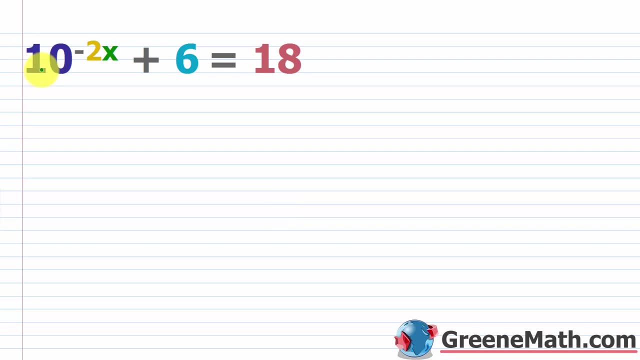 examples as we progress through the lesson. So we have 10 raised to the power of negative 2x, and then we have plus the 6, and this is equal to the number 18.. All right, so how could we solve this? Let me just rewrite it. So 10 raised to the power of negative 2x, then we have again plus 6,. 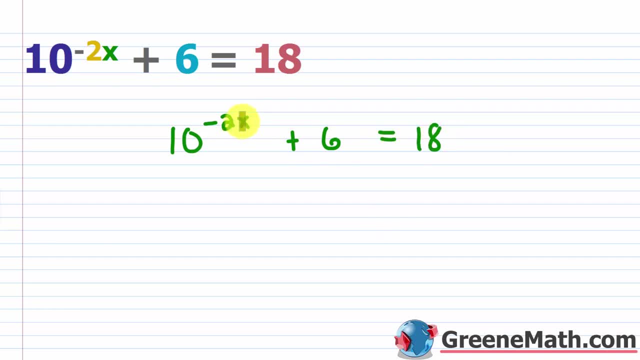 and this equals 18.. Well, the first thing you want to do if you're solving for x, you want to isolate the term that contains x in it. So this guy right here is the term that contains x in it. So to isolate that, I would just subtract 6 away from both sides of the equation. So that's the. 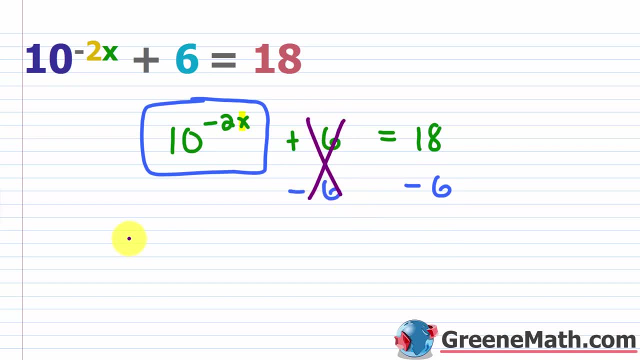 very first thing you want to do. So this cancels All right. so now, on the left, I have this: 10 raised to the power of negative 2x, and this is equal to 18 minus 6, is 12.. Now, from this point- here's where you have to think about your logarithms- that you worked. 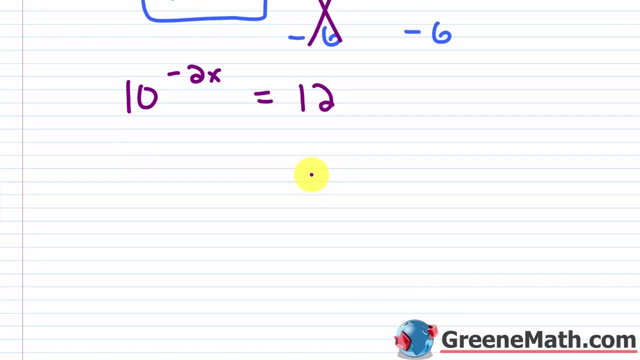 with. You know that you have the power property for logarithms and basically that allows you to take your exponent down out in front. okay, So what I want to do is use that property here so that I can get this guy to come down. okay, So if I take the log of the left side, 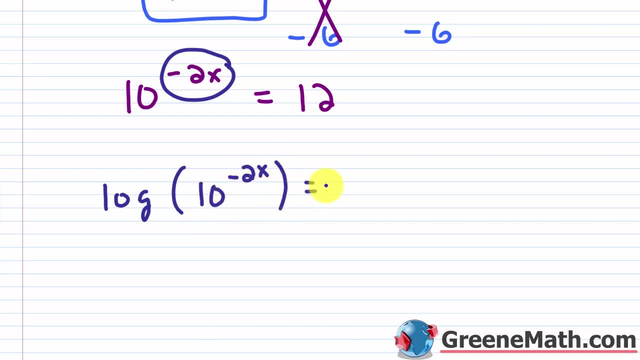 and I also take the log of the right side to make that legal. what's going to happen is from my power property. this guy right here can now come out in front, okay, So let's scroll down and get some room going and we'll see this real fast. So we're. 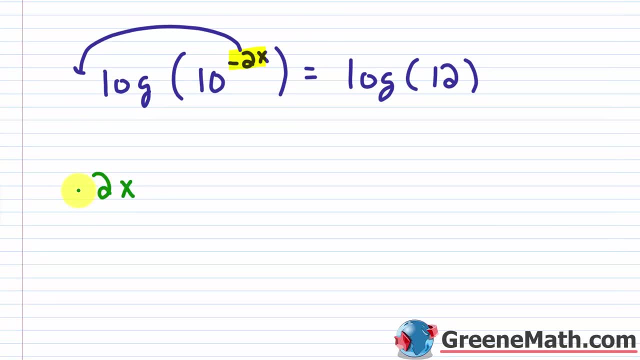 going to have our negative 2x out in front. We'll make that negative just a little bit better and then times this log of 10.. Now, this is 1, and I'll cancel that in a minute. I want to explain. 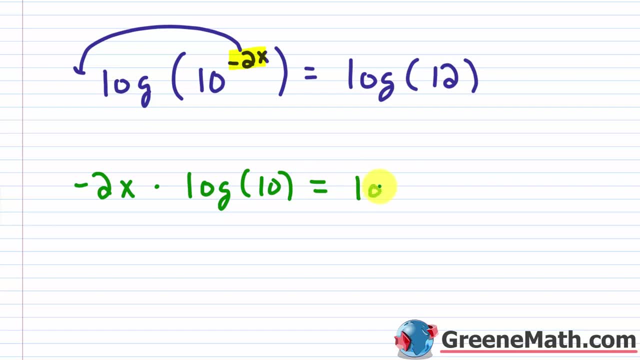 why it's 1.. I think most of you know that already, but this is equal to log of 12.. Now this is 1, so you can just cancel and put 1.. The reason it's 1 is remember, when you have log of something you don't show a base. It's. 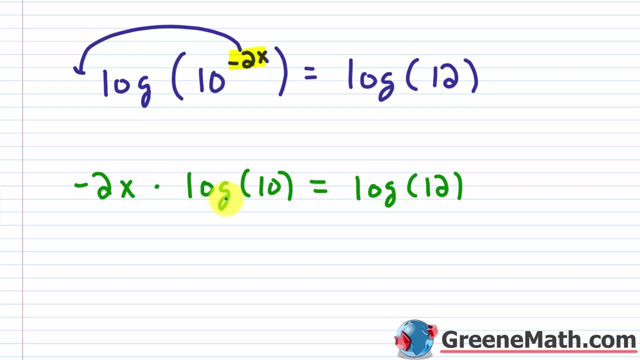 because you have the common logarithm, The base is understood to be 10.. So if I showed you that you had log base 10 of 10, again, what is this? This is equal to 1, because 10 to the first power. 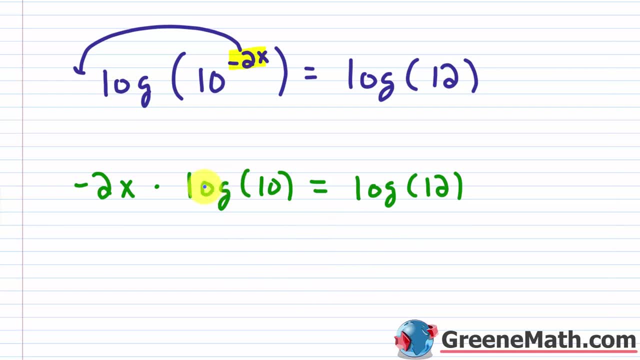 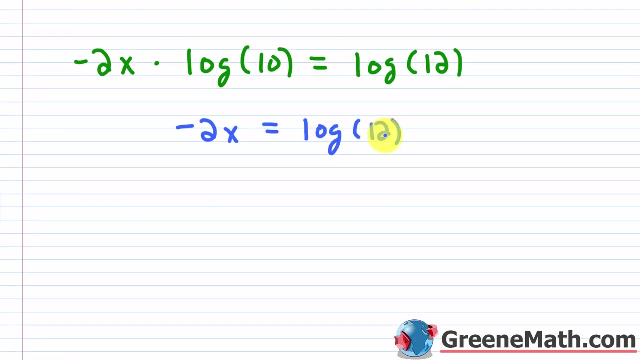 gives me 10.. So if this is 1, then really this left side is just negative 2x, because negative 2x times 1 is just negative 2x. And now this is equal to log of 12, and once we get it to this point it's really really simple. Log of 12 is just a number. 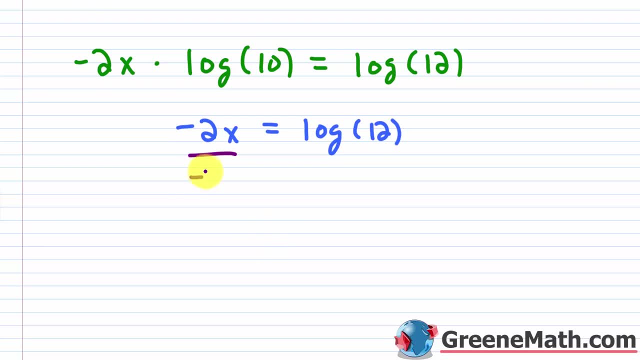 so don't let that scare you. Basically, all you want to do is divide both sides by negative 2, just like we've always done. okay, to isolate x, And so we know that this right here is going to cancel, and I have x by itself and it equals my log of 12 over my negative 2.. Now this is the. 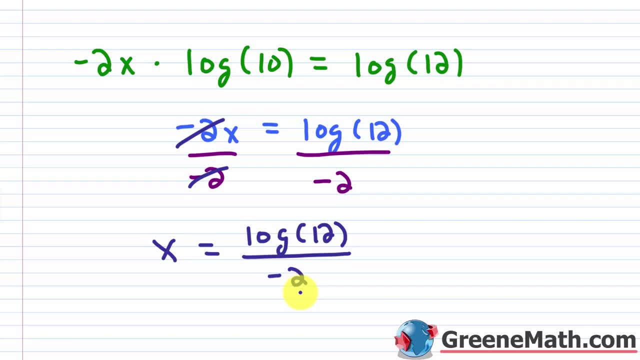 answer. if you don't want to give an approximation, If your teacher says, hey, I want the exact value, then you give this. Now, if you wanted to approximate this using your calculator, that's fine too. Generally speaking, you're going to have some specific decimal place that you're going to want to round to. 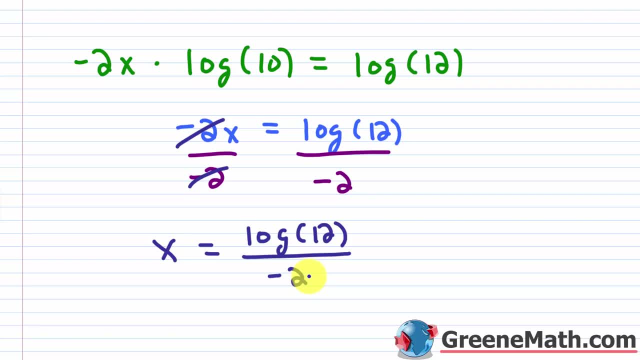 and the teacher will let you know that in your assignment. So I'm going to punch this up on a calculator and I'm going to get about, and I'm going to use my approximate sign there, So negative, and then I'm going to say 0.5396.. And again I'm rounding this guy and again I'm using the. 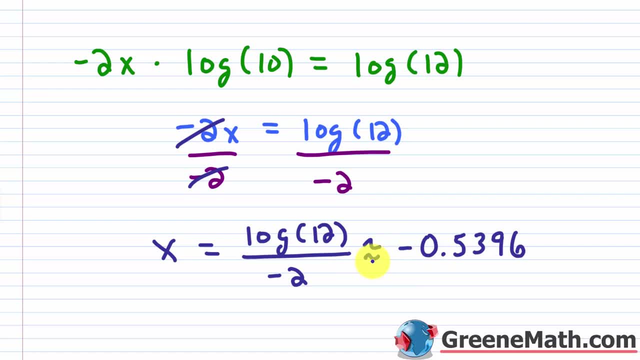 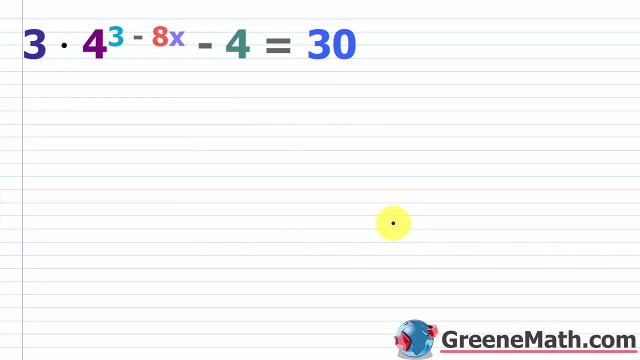 approximation symbol there To show that it's a rounded amount, it's an approximation. It's not the exact amount, but it's pretty close. All right, let's take a look at a harder example, or I'd say a more tedious example. So now we have 3 multiplied by 4, raised to the power of 3 minus 8x. Then we have 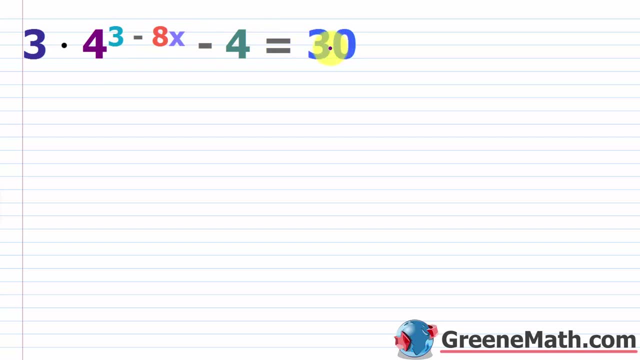 minus 4, and this is equal to 30. So again, the first thing I want to do, since x is here, I want to isolate this guy. okay, So to do that, I have multiplication here and I have subtraction here. Let me add 4 to both of them. So I'm going to do that. So I'm going to do that. 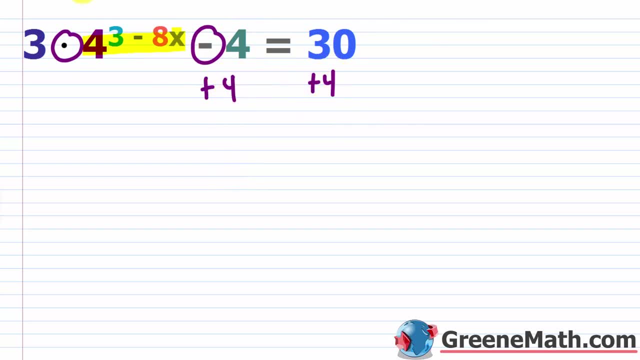 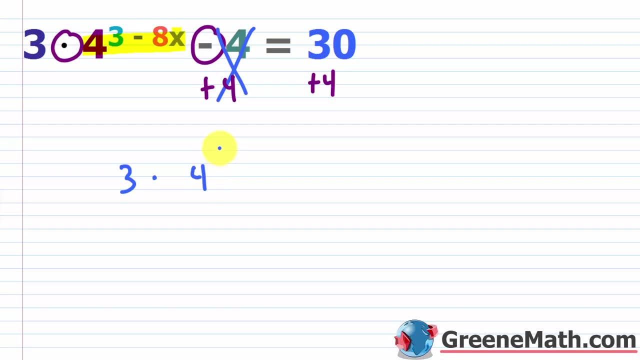 the left side. now I have 3 multiplied by 4, raised to the power of 3 minus 8x, And this equals 30 plus 4 is 34.. Okay, So from here again, if I'm trying to isolate this guy, well, what do I have? 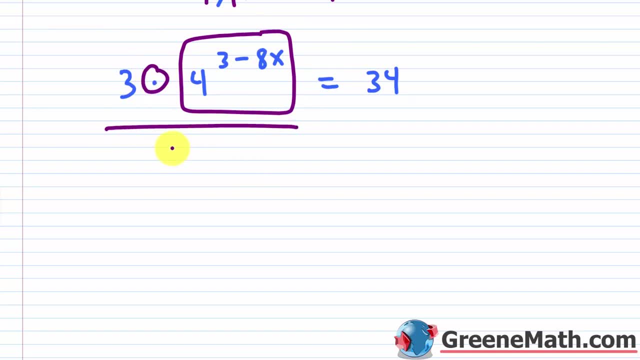 I have multiplication here, So to undo that, I'm just going to divide both sides by 3.. And now this is going to cancel here, And what I'm left with on the left is what I wanted to isolate. So I have 4 raised to the power of 3 minus 8x, And this equals my 34. 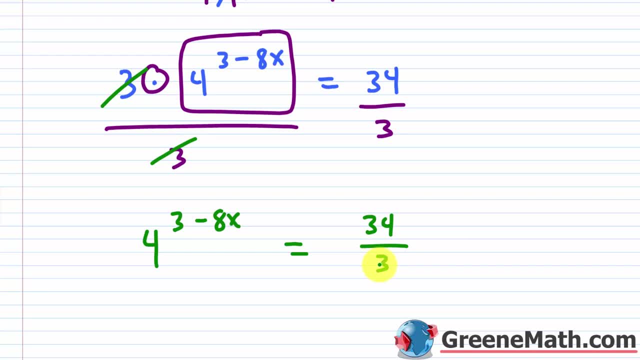 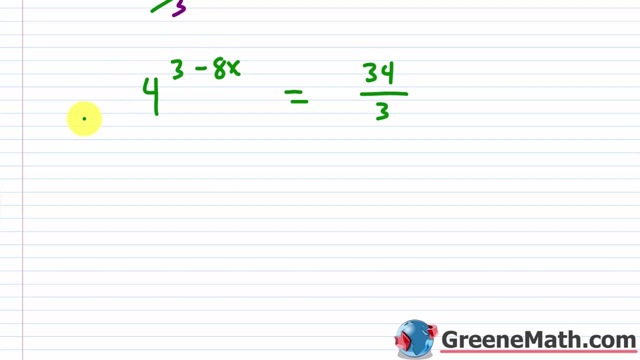 over 3.. Okay, So from this point, I've got to find out how I can get this variable down, okay, And to do that again we're going to use our power property for logarithms. So I'm just going. 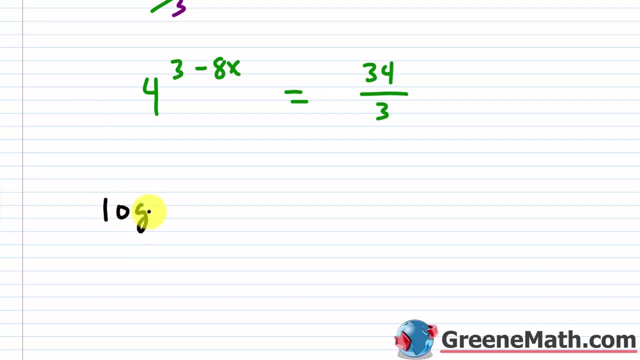 to take the log of both sides. So I'm just going to go: log of 4 raised to the power of 3 minus 8x, And this will be equal to log of. you have your 34 over 3, or 34 thirds, if you want to say it that way. Okay, So from here. 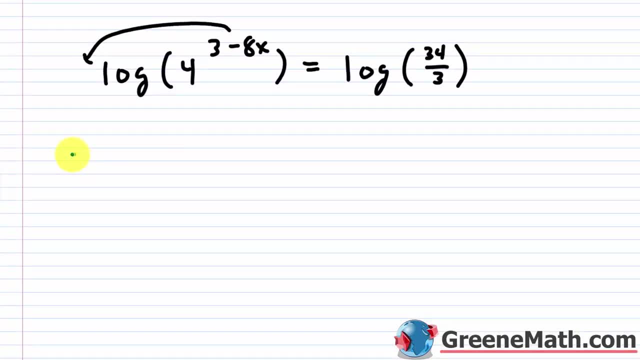 this can come down right from the power property. So you have your 3 minus 8x times your log of 4.. Now I want to caution you against something: It's very important that you use parentheses here, because this is a quantity- 3 minus 8x- and it's being multiplied by 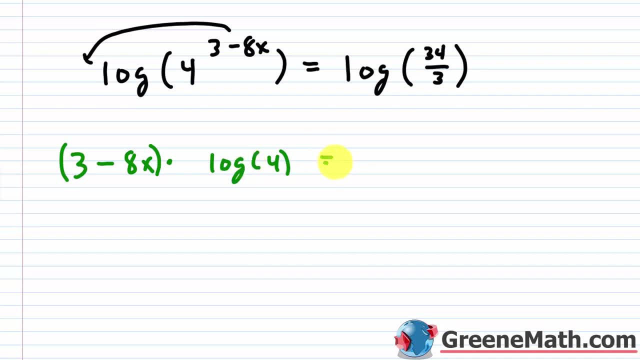 log of 4, which is just a number. So we'll say this is equal to log of again 34 thirds. Now let me make this a little better, a little cleaner. So 34 thirds, Okay. So at this point you can do this two different ways. You can use your. 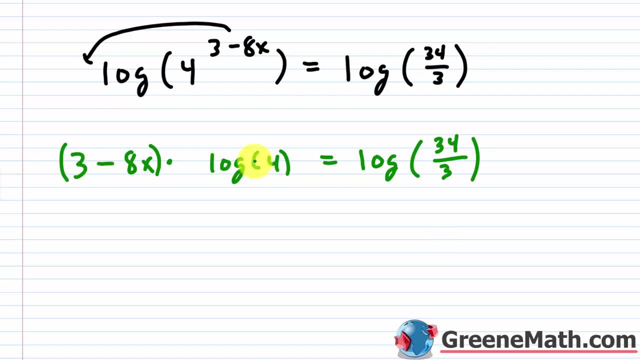 distributive property here. So you can multiply log of 4 by 3, and then log of 4 by negative 8x. You can do it that way, Or you can get rid of this guy right now by dividing both sides by log of 4.. 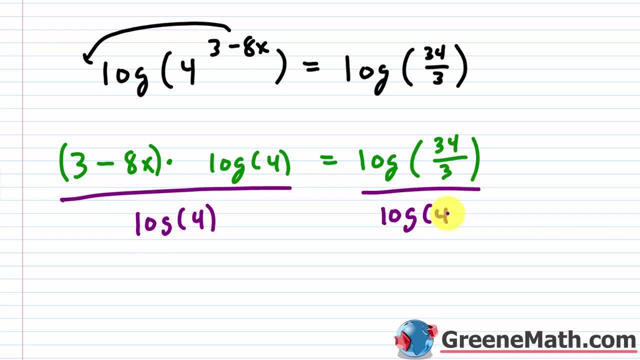 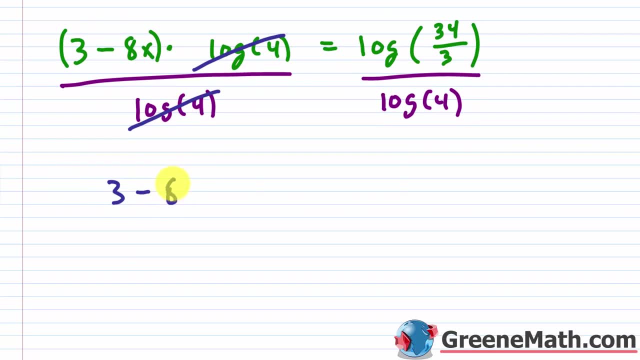 And that's what I'm going to do. You'll get the same answer either way, So it doesn't really matter. So let's go ahead and cancel this with this And let's scroll down now, So I'll have 3 minus 8x And you can drop the parentheses- You don't need them anymore- And then this is equal. 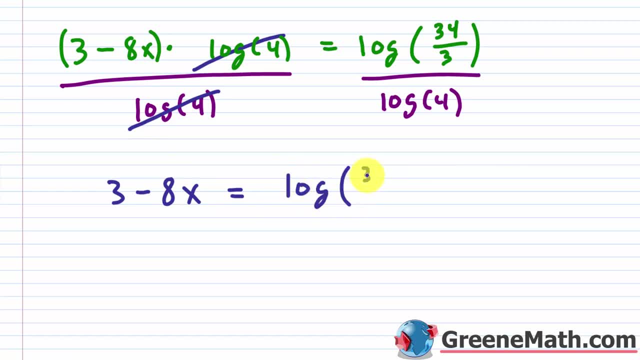 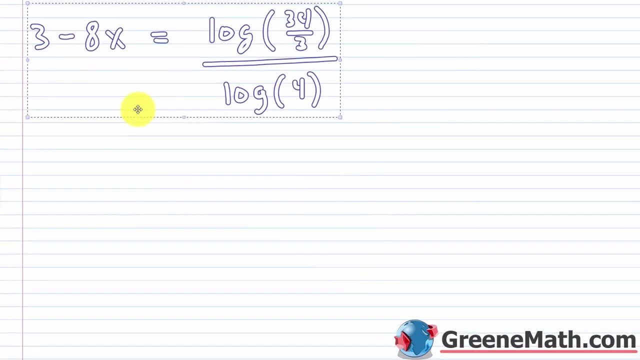 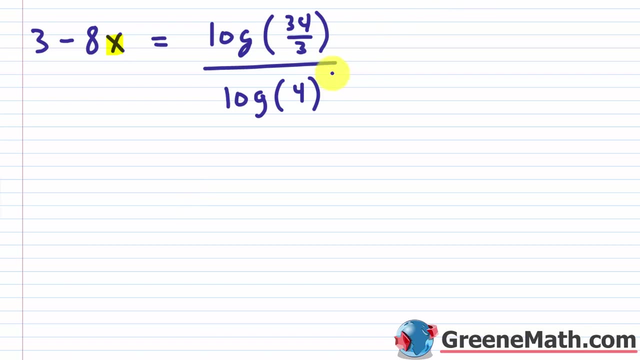 to: you've got your log of, you've got this 34 thirds, And then this is divided by log of 4.. All right, So from here, what we need to do is again isolate this x. So I'm going to start by 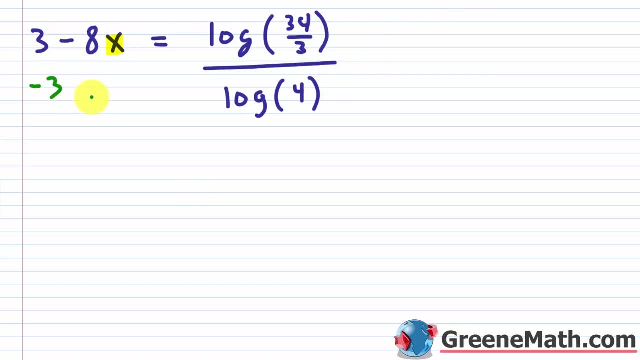 subtracting 3 away from the power property, And then I'm going to do this. So I'm going to subtract 3 away from each side of the equation. So I'm going to subtract 3 away from here, That's going to cancel. I subtract 3 away from over there. So now I have what I have: negative 8x. 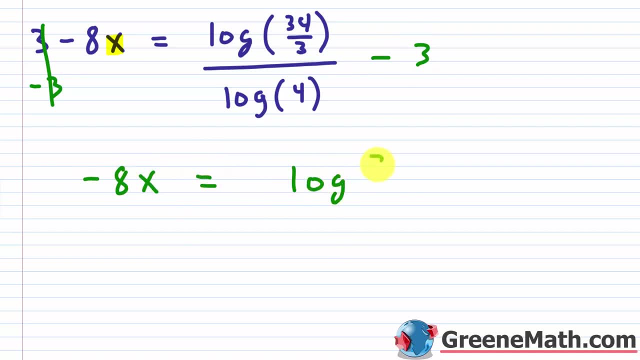 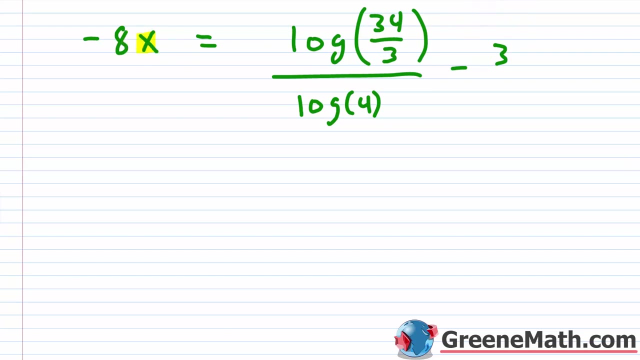 is equal to this log of 34 thirds, And this is over my log of 4.. And then over here I have minus 3.. Okay, So to finish things up, I'm just going to again try to solve for x And to do that. 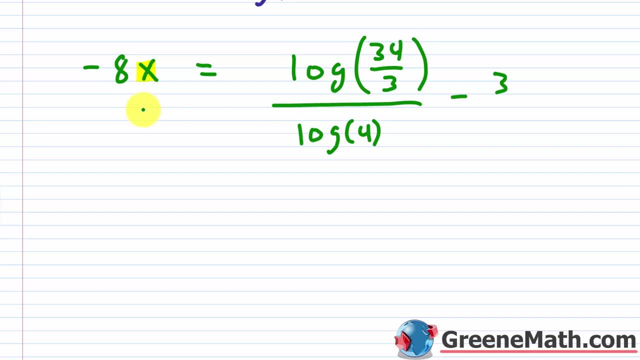 just like we've been doing forever. I want to divide both sides by negative, Negative 8.. But really an easier way to think about this here, because we have a fraction involved. I'm going to multiply both sides by negative 1- 8th. Okay, So that would be the same. 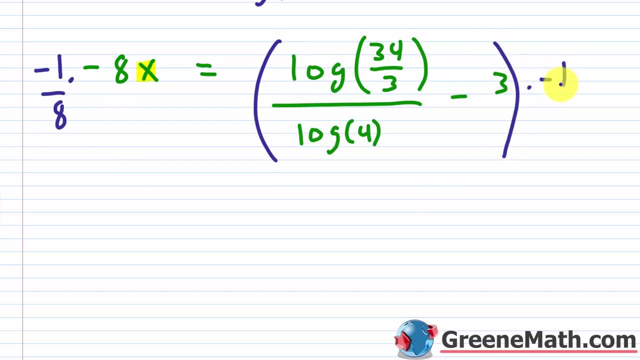 thing: Make sure you use parentheses here. So times negative: 1: 8th. This, of course, is going to cancel, And on the left you just have your x that you're looking for. On the right, I'm going. 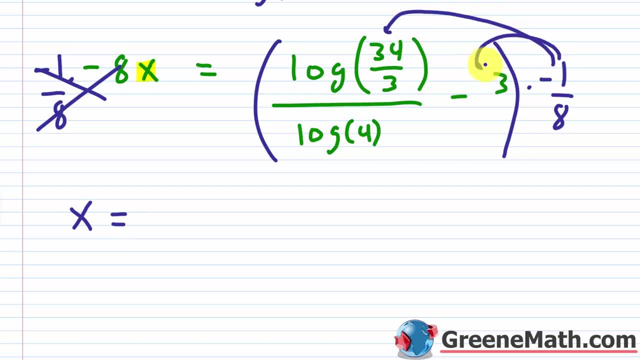 to distribute this to each, And so what's going to happen is, for the first one, I'm going to have the negative of log Of 34 thirds over. you're going to have this 8 out in front times log of 4.. Okay, Then what do we? 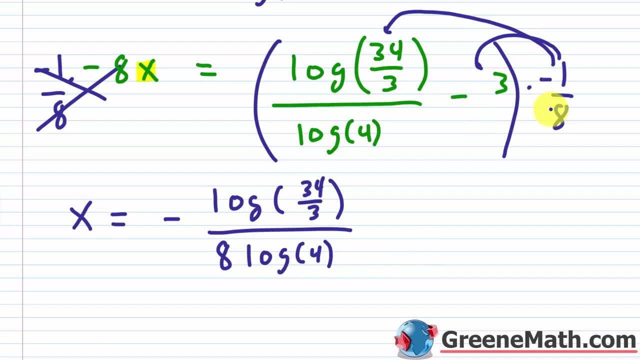 have? We basically have negative 3 times negative, 1- 8th. So that would be what. That would be plus 3 8ths. So this is going to be your answer Again, if you don't want to give an approximation. 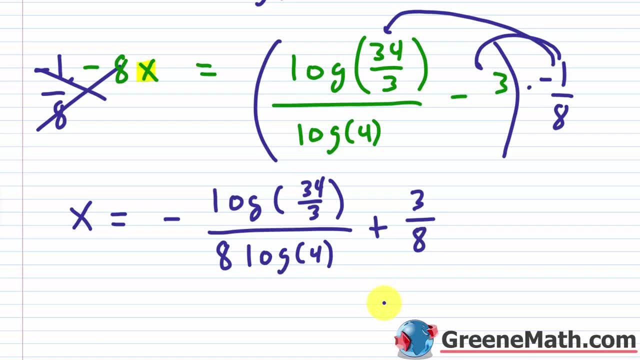 you would basically say that x is equal to the negative of log of 34 thirds, over 8 times log of 4, plus you have your 3 8ths. Now, if you wanted to give an approximation, you're going to get. 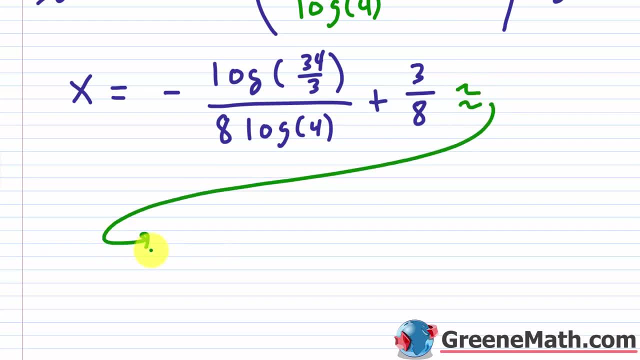 about. okay- and I'm going to bring this down here because I'm going to run out of room- We're going to say 0.1561.. So again, here's your approximation And here's your exact value. Again, the negative log of 34 thirds over 8 times log of 4 plus 3, 8ths And then, as an approximation, 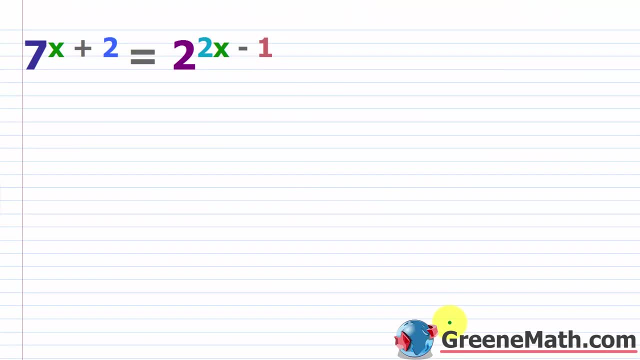 0.1561.. All right, Let's take a look at another one. So we have 7 raised to the power of x plus 2 is equal to 2 raised to the power of 2x minus 1.. So this one is a little bit quicker to do. 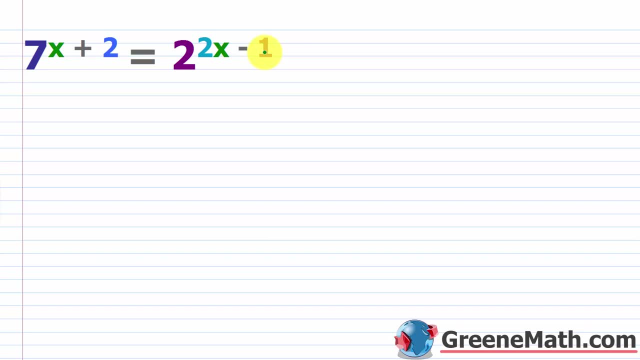 but you do have some things that kind of trip you up on this. There's nothing really to do other than to take the log of both sides to start, because you've got to get these guys down. Okay, You can't solve it the way it is, So you go. log of 7, raised to the power of x plus 2.. And this: 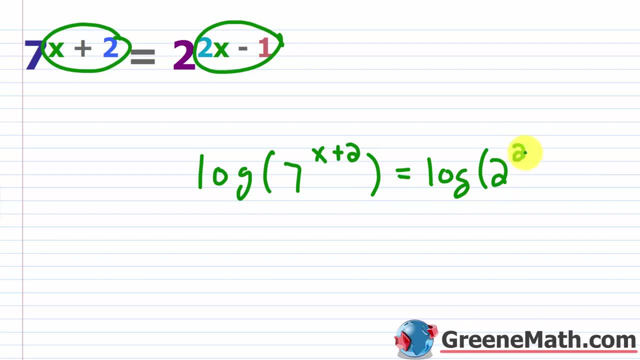 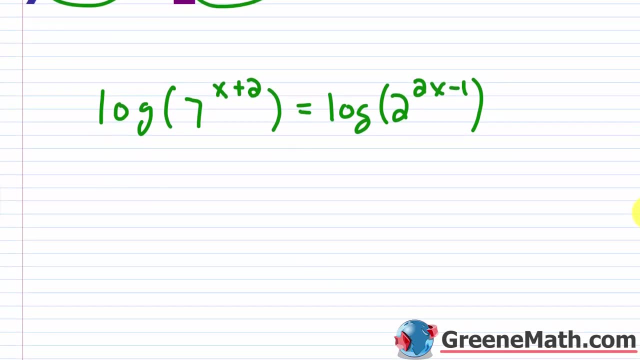 equals 2.. Log of: you have 2 raised to the power of 2x minus 1.. And let me slide this down so it's in the middle of the screen. And so now we know that those exponents can come down So legally. 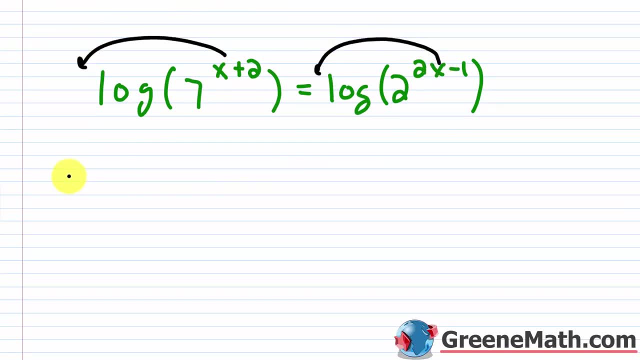 I can say that this is what This comes down. This comes down. So we have this: x plus 2.. Again, this is a quantity, So I'm going to use parentheses. times log of 7 equals this comes down, So the quantity 2x minus 1 times log of 2.. So again, here's where I'm going to. 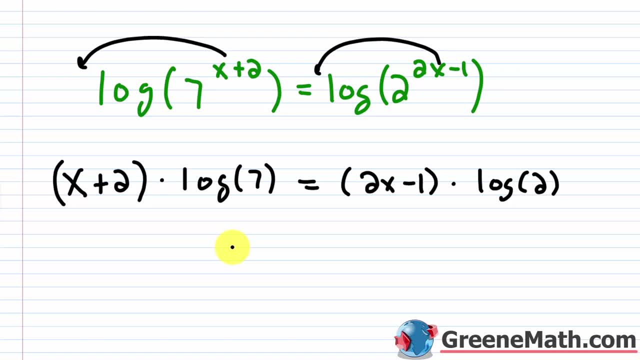 use my distributive property. you've got to get everything with an x on one side so you can factor that out and solve for x. So I'm going to go and distribute this to each term here, So I'm going to have x times log. 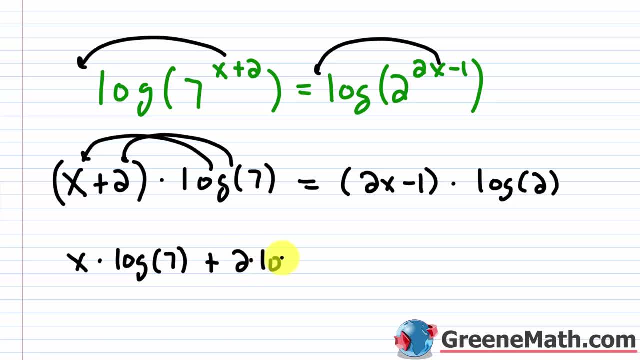 of 7, then plus 2 times log of 7. And this equals over. here I'm going to have 2x times log of 2.. Let me slide this down so I don't run off the screen, And then I'm going to have minus 1 times. 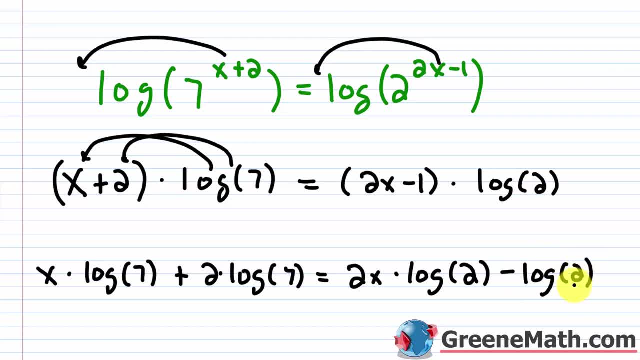 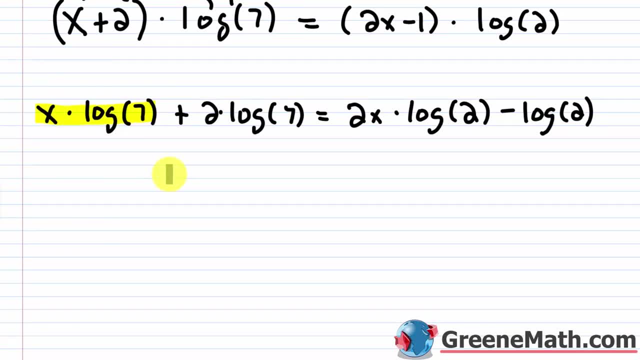 log of 2, which is just log of 2.. Okay, so now what I want to do is get all my terms with x involved to one side. Okay, so I'm going to have this guy right here and this guy right here. 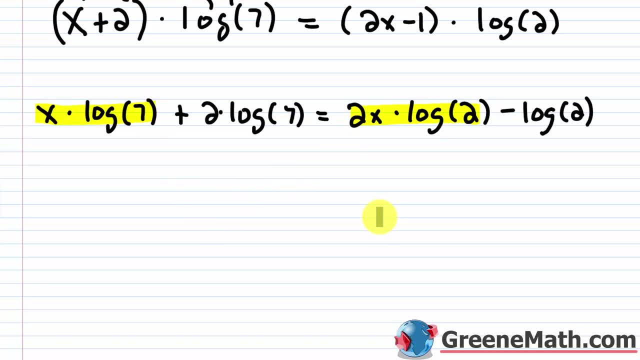 everything else you want on the other side. Again, the reason you're doing this is so you can factor the x out and then solve for it. So what I'm going to do is subtract 2 times log of 7 away from each side of the equation, And I'm going to subtract 2x. 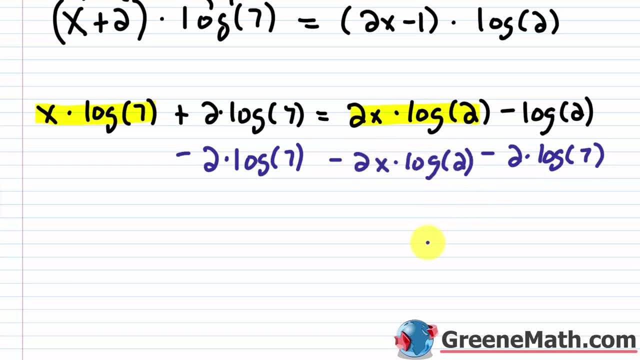 times log of 2, away from each side of the equation. So let me do that over here. So minus 2x times log of 2.. Okay, And so this guy's going to cancel. and this guy's going to cancel, And what? 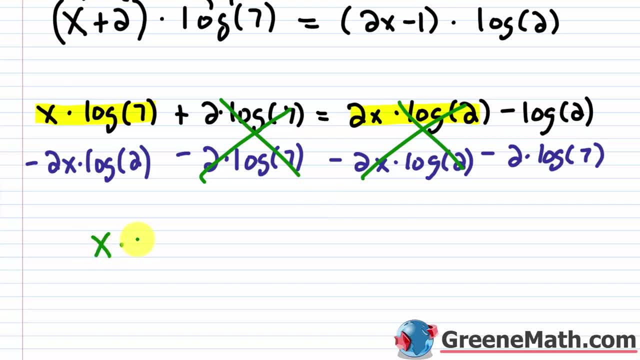 do I have? Well, my new left side is going to be x times log of 7 minus 2x times log of 2.. Let me scooch this down a little bit And this will be equal to my right side. will be what? 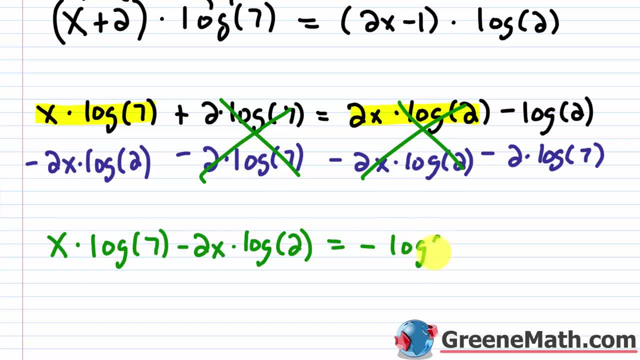 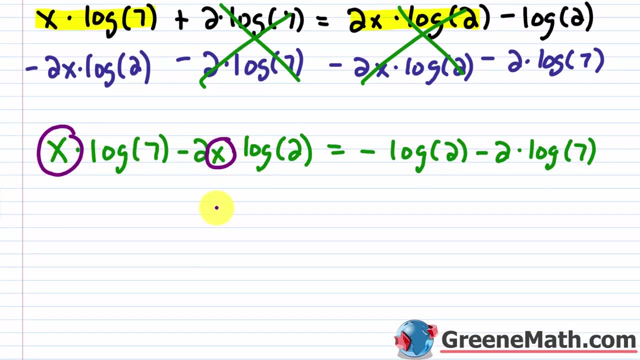 I'm going to say that I have the negative of log of 2 and then minus 2 times my log of 7.. Okay, So how do I solve for x? Again, I want to just think about factoring it out. So if I factor out an x from here and here, what would that leave me with? So this comes out. So I 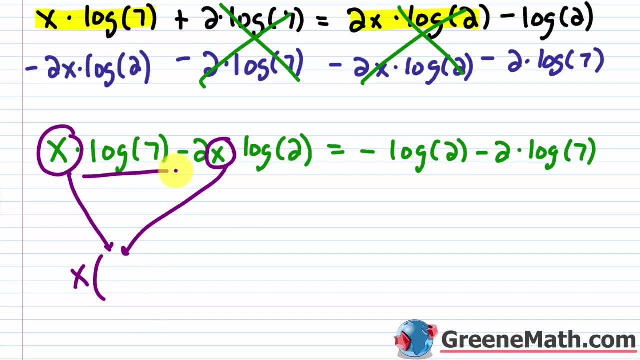 have x out in front And inside the parentheses. I have the log of 7 minus. you're going to have this 2 here times this log of 2 here. So I would have log of 7 minus 2x times log of 2 here. 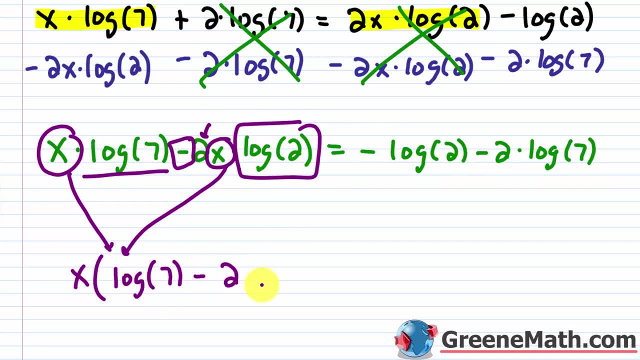 So I would have log of 7 minus 2x times log of 2.. Okay, And let me put some closing parentheses there, And this will be equal to again over here. this isn't going to change. So we have negative log of 2 minus 2 times log of 7.. All right, So now how can I get x by? 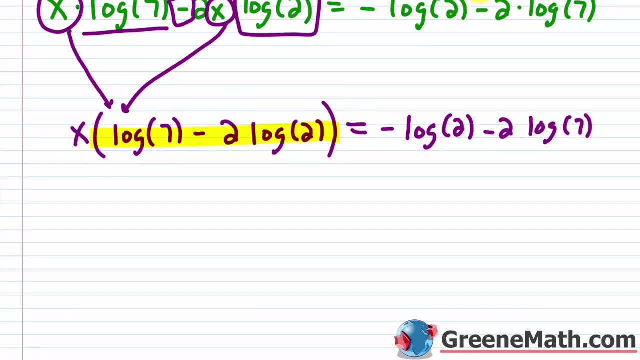 itself. Well, this guy right here is just multiplying x, So all I have to do is just divide both sides. so divide by log of 7 minus 2 times log of 2 on both sides. So log of 7 minus 2 times log of 2.. 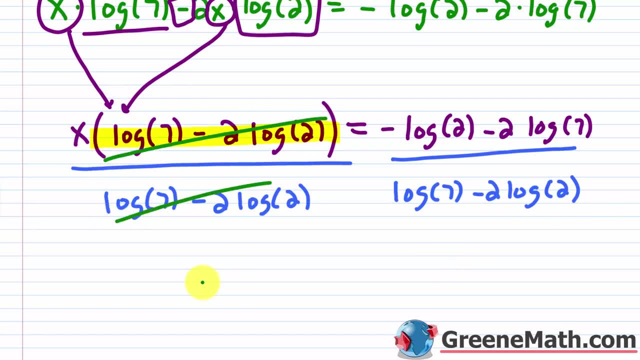 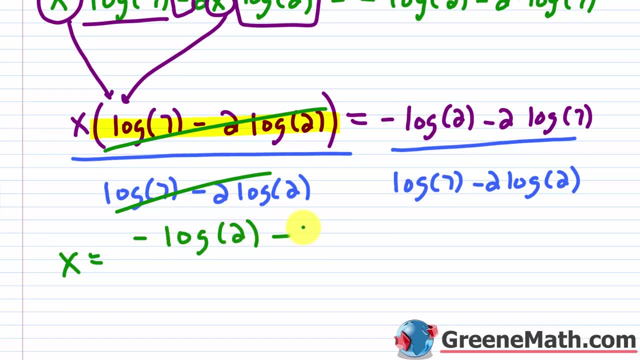 And what do we get? Well, this cancels, So that's done. We get. x is equal to: we'll have that negative log of 2 minus 2 times log of 7 over log of 7 minus 2 times log of 2.. 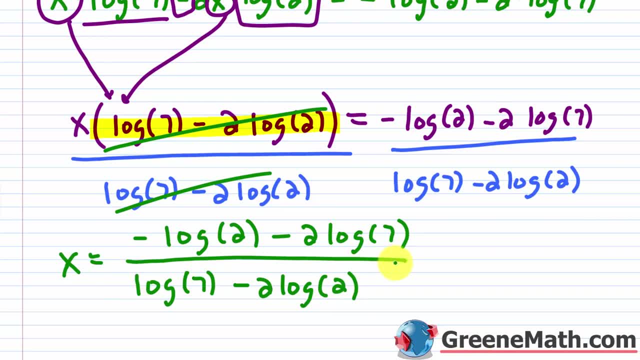 So again, this is your exact answer. If you want to give an approximation, I'll just give one here as an approximate value, And let me make that sign a little bit better. So you punch that into your calculator, you're going to get about negative. 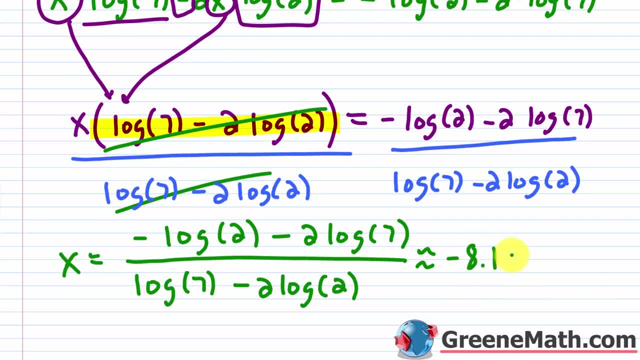 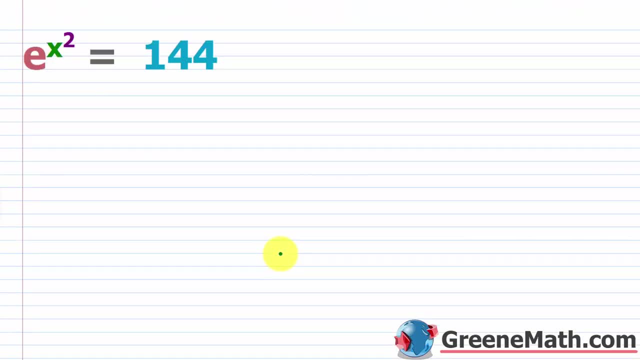 8.1931.. Again, that's just an approximation. All right, Let's go ahead and take a look at another example. So we have e raised to the power of x squared equals 144.. So for the previous examples I used the common logarithm, So I put the number such that we're going to have x squared. 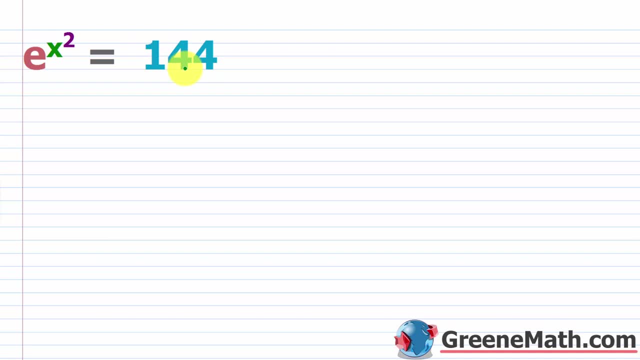 and what I know is that those are the values for x squared. So we have e raised to the power of x squared equals 144.. So for the previous examples I used the common logarithm, So Commezor, or again the logarithm with a base of 10, that's the log key on your calculator. Now I'm going to 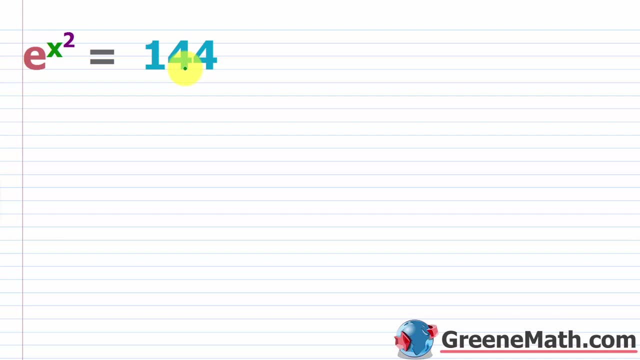 use the natural logarithm, the LN key, on your calculator, because whenever you deal with this special number E, remember, if you type LN for the natural logarithm into your calculator and then you hit E as the argument, you're going to get a value of one right, Because this LN 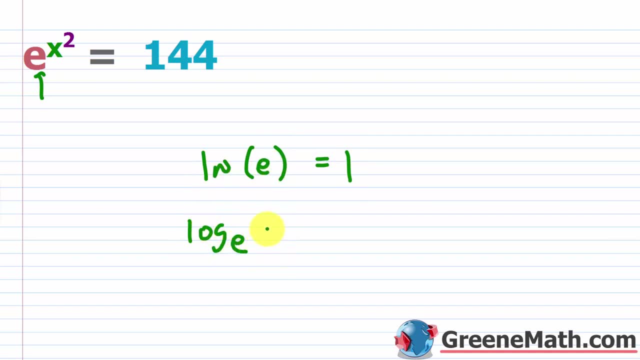 this represents a log with a base of E, And then, if it's of E, this is what E to the first power gives me E, So that's why this has a value of one. So what I'm going to do here is I'm going 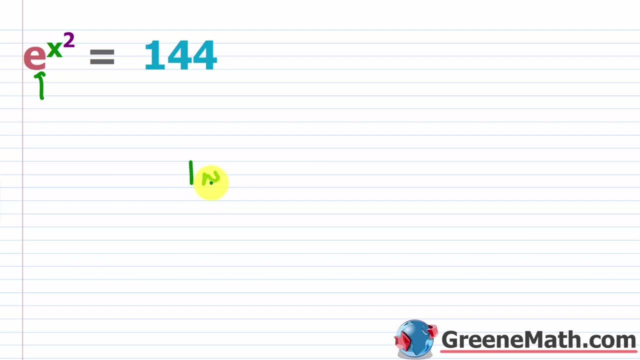 to use the natural log for each side. So this LN is how you want to write, that of E raised to the power of X squared, And then again for the natural log on this side, write the LN and then of 144.. And so this can now come down. So I'll say I have X squared times if I have the natural log. 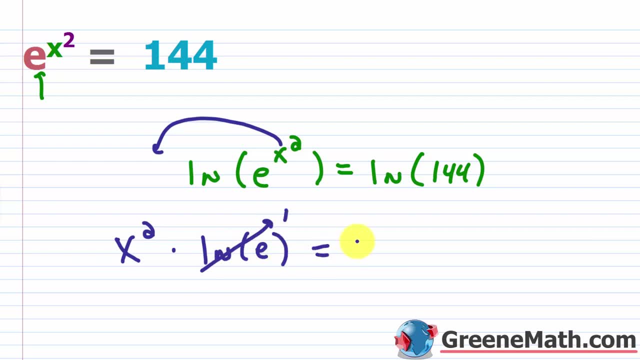 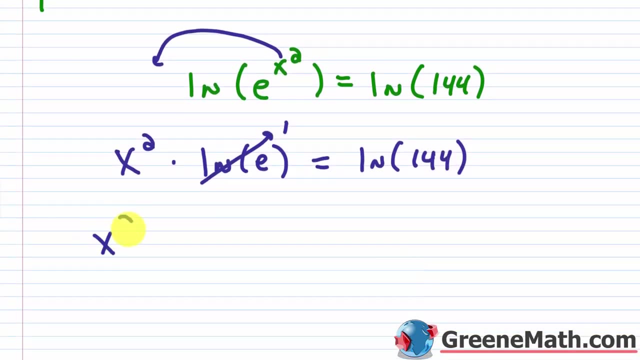 of the number E. this is one, okay, And this equals again the natural log of 144.. Okay, So from this point, what do I have? I have that X squared is equal to the natural log of 144.. 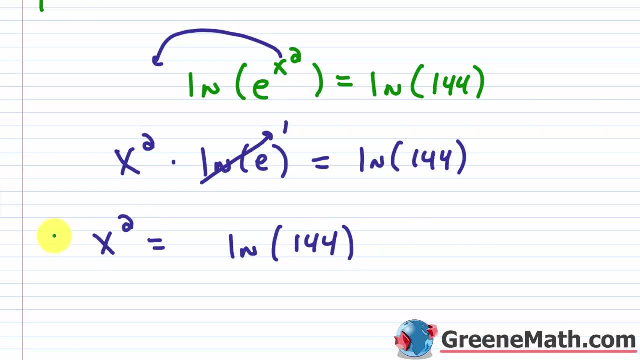 And how can I get X by itself? Well, I just take the square root of each side. So I take the square root of this side, Let me make that better- So the square root of this side, and then remember, you got to do your plus or minus the square root of this side. Okay, So we know that. this on the 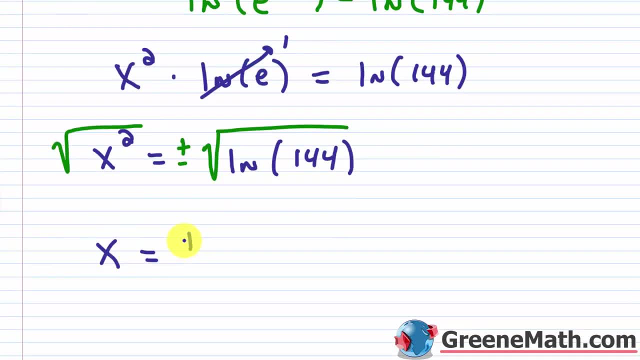 left is just going to be X now, And this equals plus or minus the square root of this natural log of 144.. So I'm going to take the square root of this side and I'm going to take the square root of 144.. Once again, this is going to be the exact answer. So you have plus the square root of the. 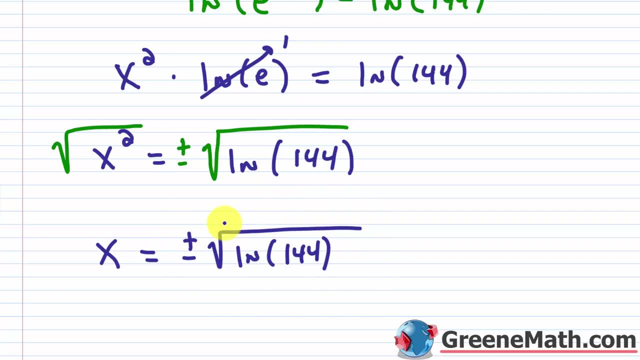 natural log of 144, and then you have minus or the negative of the square root of the natural logarithm of 144.. So that's the exact value. If you want an approximation, okay, you can type this into your calculator and you're going to get approximately plus or minus, we'll say 2.2293.. 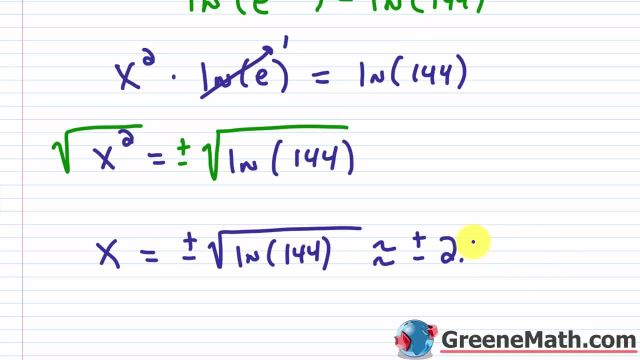 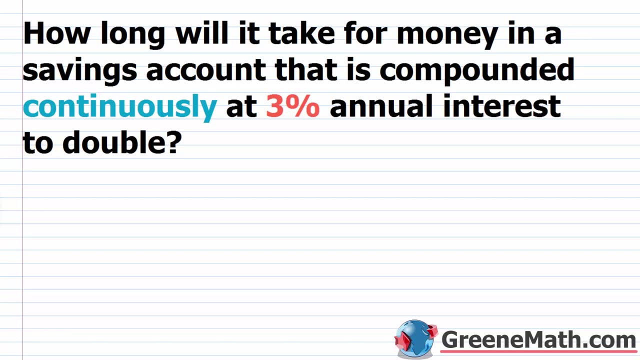 Let me make that a little bit easier. So I'm going to take the square root of this side and I'm going to. So 2.2293 is a good approximation for this. All right, What I want to do now is look at a typical. 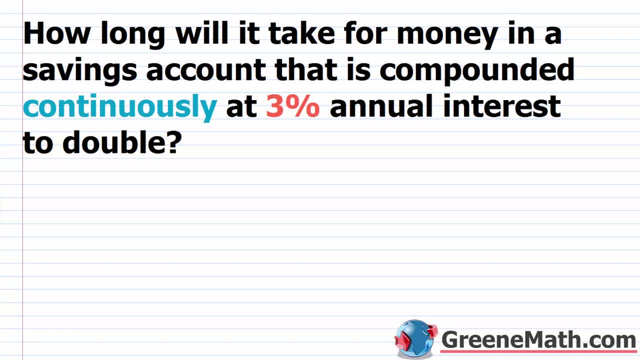 word problem that you're going to see in this section And basically it goes like this: We have: how long will it take for money in a savings account that is compounded continuously at 3% annual interest to double? So this is a very simple word problem to solve, But a lot of times 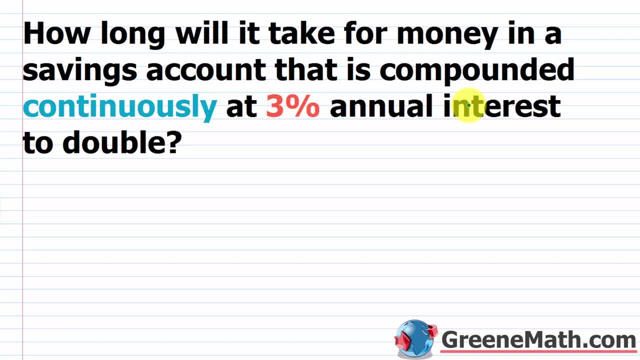 if you haven't seen it before, you might get tripped up. So the first thing is to remember the formula for the continuous compound interest. So that's: the A is equal to P times the special number E, raised to the power of R times T. 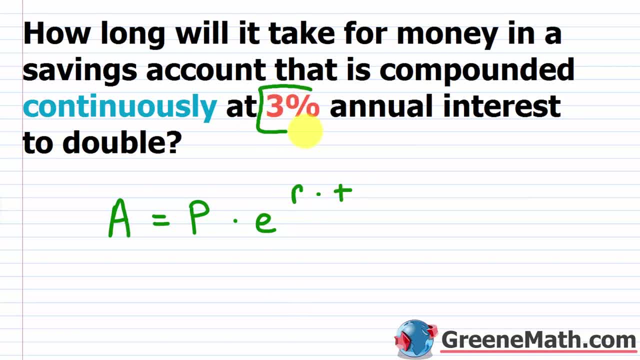 So again, the R is the rate as a decimal. We have that here. It's 3%, So you're going to plug that in there. So let me just do that now. So let me put this as 0.03.. And then times again that T. 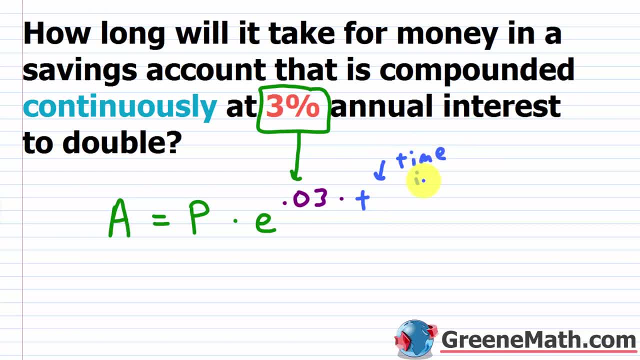 this is your time in years. your time in years, Okay. So remember that. Now, when we think about the rest of this, we have P, which is the principal, and we have A, which is the account balance in the future. You could say the future. 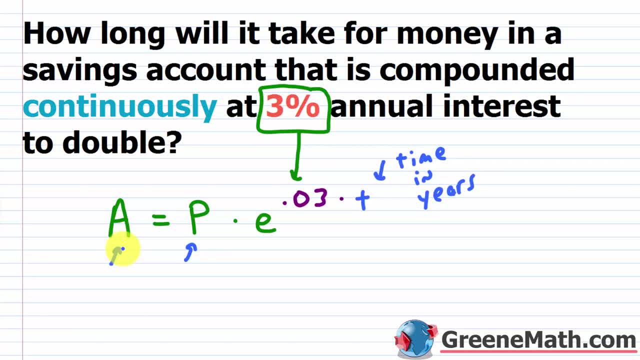 value of the account. So typically for these problems, you're given an interest rate, you're given a time in years and you're given a principal, a starting amount. You don't really have any of that here, Okay, So that's what trips people up. What you have to realize is that you're 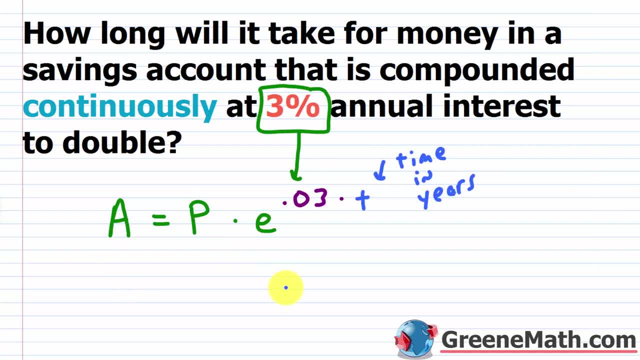 trying to figure out how long it's going to take for the money to double. So you're going to be solving for T here, Okay, And in order to get A and P to behave in this problem, you really have to think about writing A in terms of P, Okay. So again, you're trying to double your money. So whatever you put, 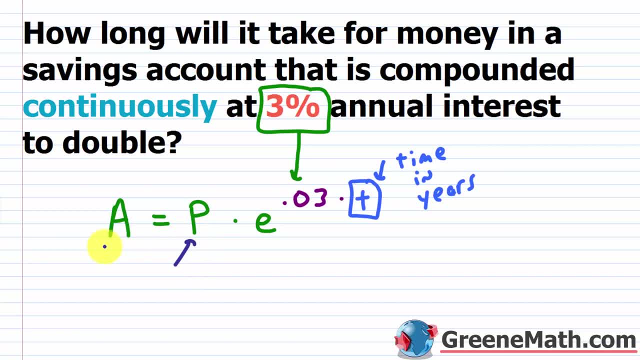 in for P. you're going to have double that for A when this happens. So this is going to be two times whatever P is. So once you realize that, once you get past that roadblock, the rest of this is super easy. You're just going to divide both sides by P And I made that a. 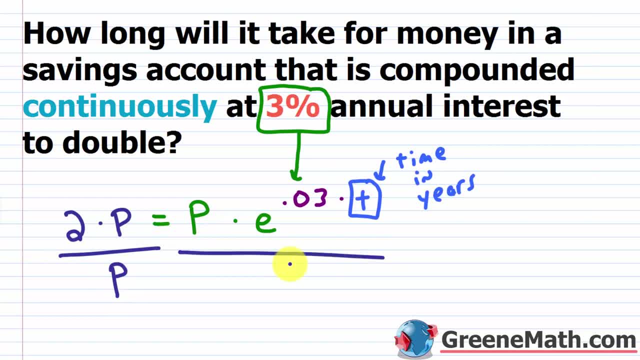 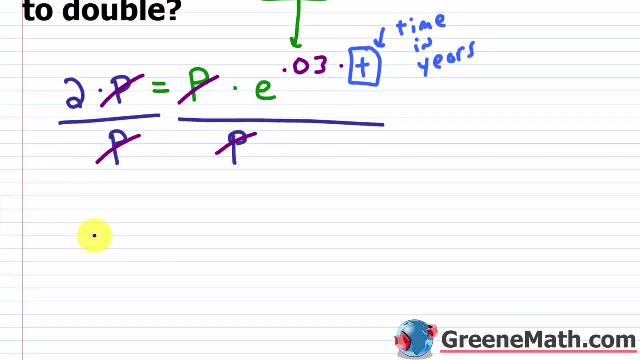 little bit easier. So you're just going to divide both sides by P, And I made that a little bit too long. So let's divide both sides by P, And we know that this would cancel, and this would cancel, And from here it becomes very, very simple. We have two is equal to E, to the power of. 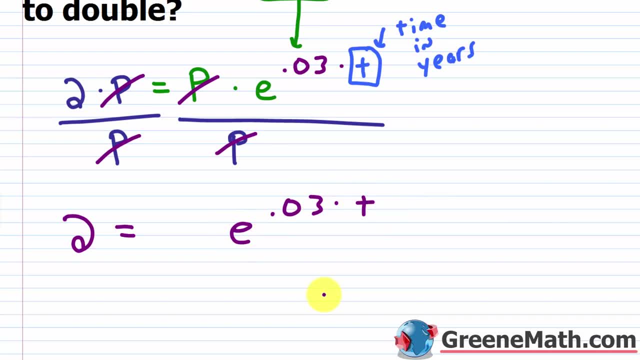 0.03 times this variable T. Okay, So from here, let me move this down a little bit. I'm going to take the natural log of each side, And the reason I'm going to do that is, again, I'm working with this special number E. 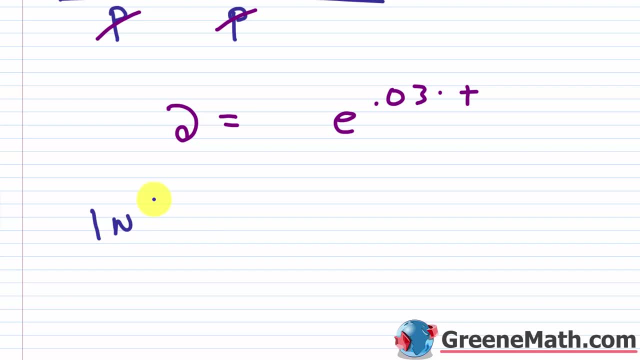 So I'm going to say: the natural log, or again use the ln of 2 is equal to the natural log of this side, which is E raised to the power of 0.03 times T. Okay, So from this point, 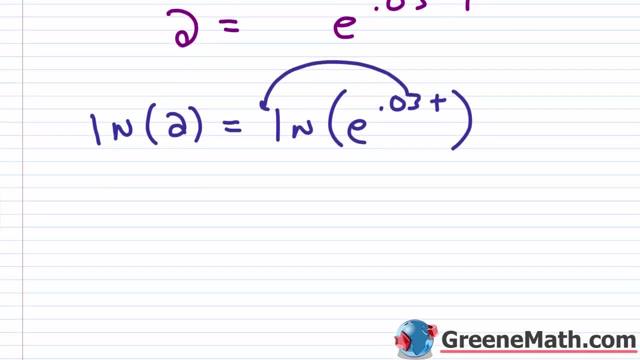 I know that this can come down, So let's come down here And we'll say what We have. the natural log of 2 is equal to my 0.03 times T, And then times what is the natural log of E. 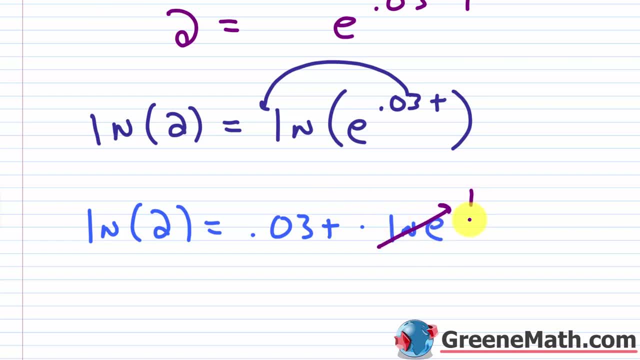 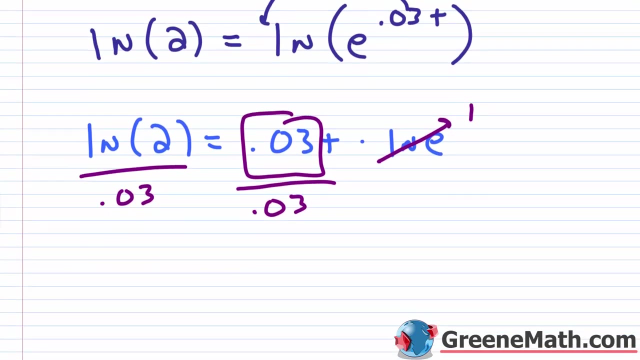 We know that this guy is 1.. Okay, So that's going to cancel. So what I have now is that T is going to be equal to what? Well, this is multiplying T. So I just divide both sides by 0.03 and I am done. So very, very simple. overall, We can say that T or the time in years, 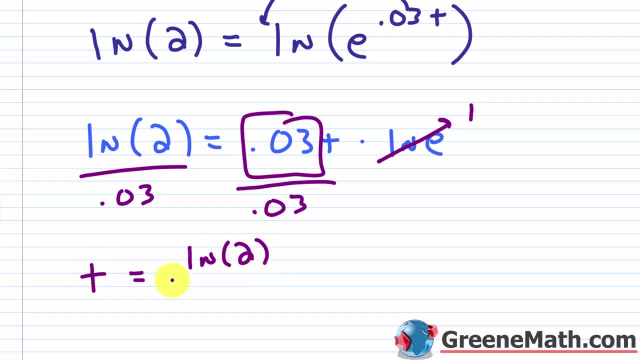 is equal to the natural log of 2 over 0.03.. Now, this was a word problem. So if you give this a question and it doesn't answer, it's basically going to be nonsense, right? You need to give an. 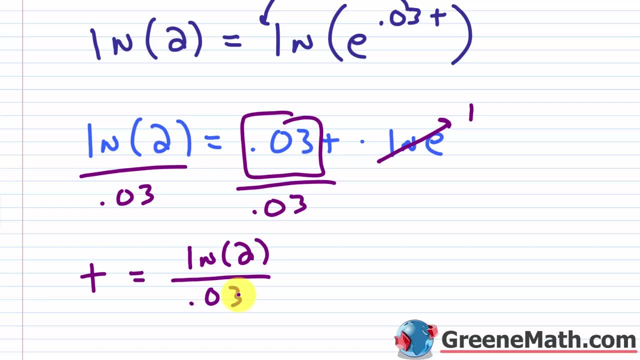 approximation here, And depending on how precise you want to be, I would round this and say that it's about 23 point. let's just go ahead and say 1, 0.. That's pretty close. Again, you can add more.